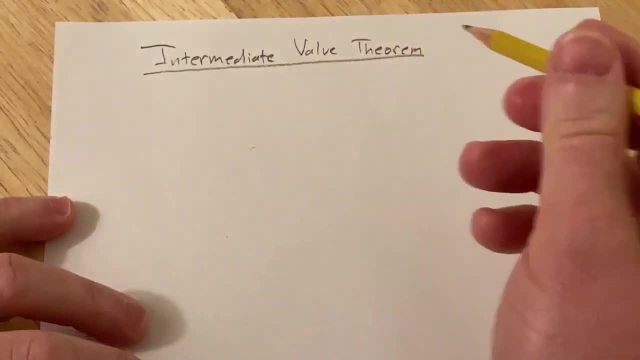 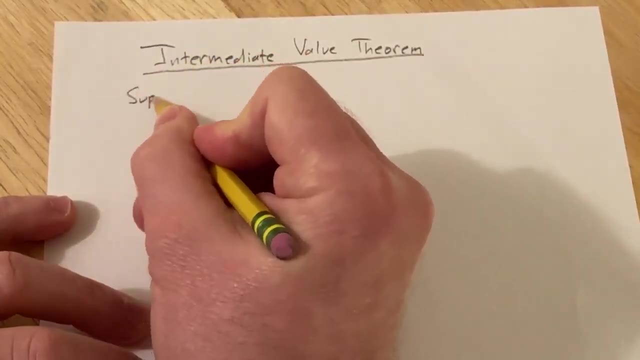 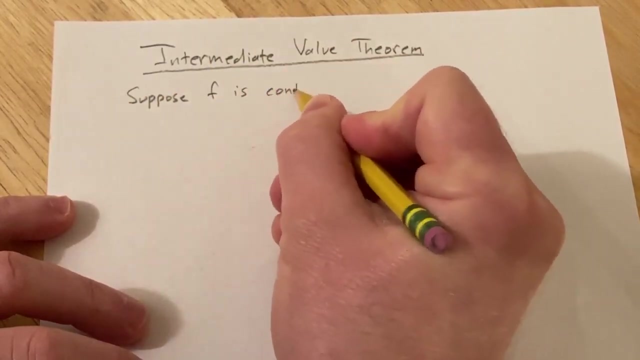 there's many ways to apply this theorem. you can apply this to a variety of problems. we're just going to pick a simple example. So the Intermediate Value Theorem says that if you have a continuous function, so suppose f is continuous. on, let's say a, b, So we have. 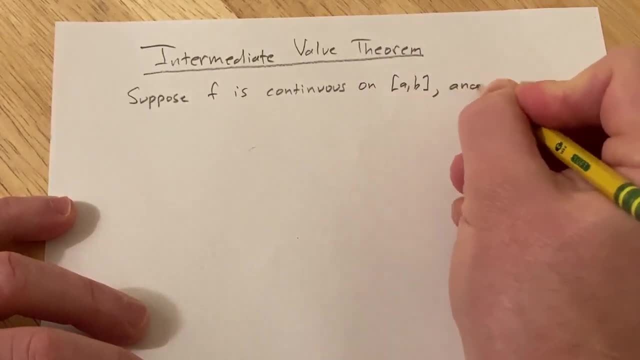 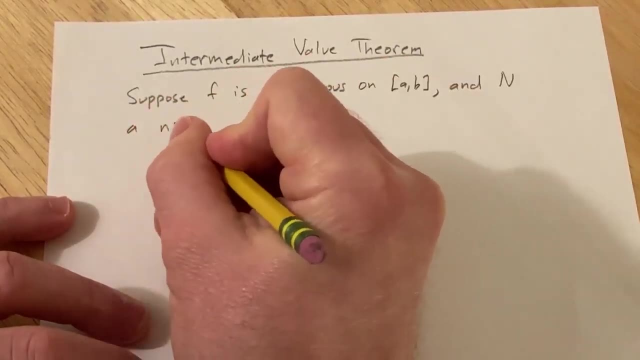 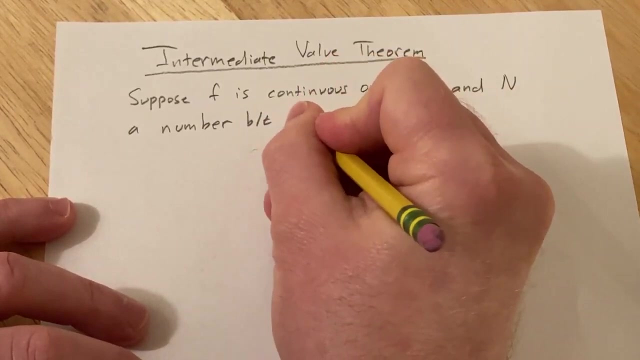 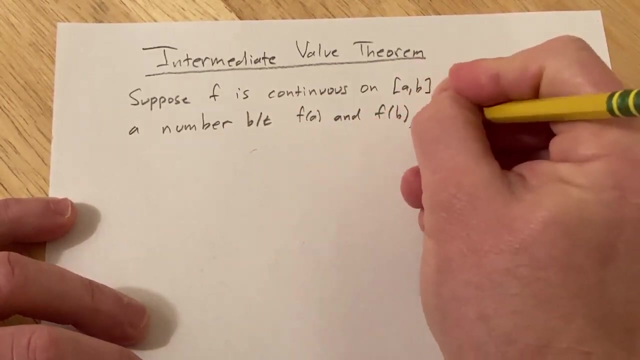 a continuous function on a closed interval, and I can use any variable. here I'll use n And n, a number. So n is some number between. that means between f of a and f of b, where f of a is not equal. 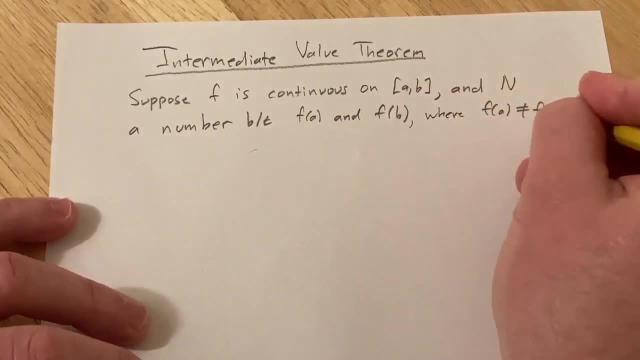 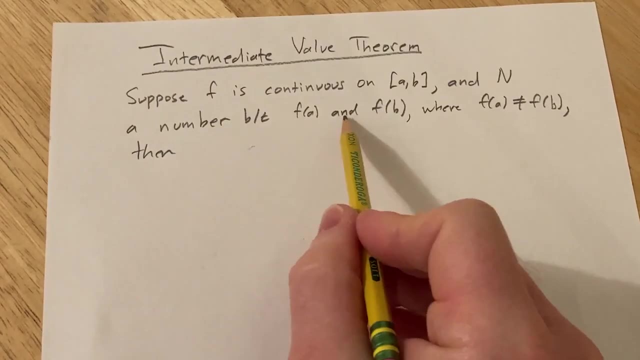 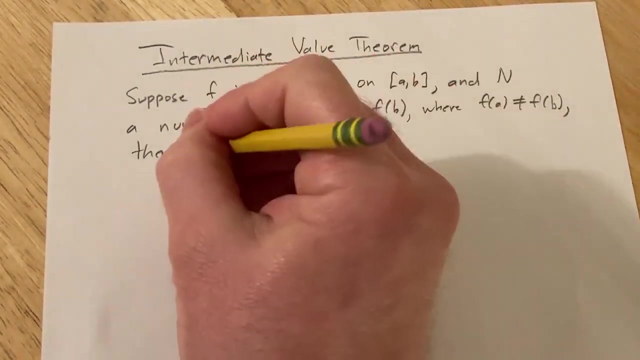 to f of b, so these are different Then. so if you have these things, a continuous function on a, b, N is some number between f of a and f of b, and these are different. so if you different, then the intermediate value theorem says there exists a number c, so then there. 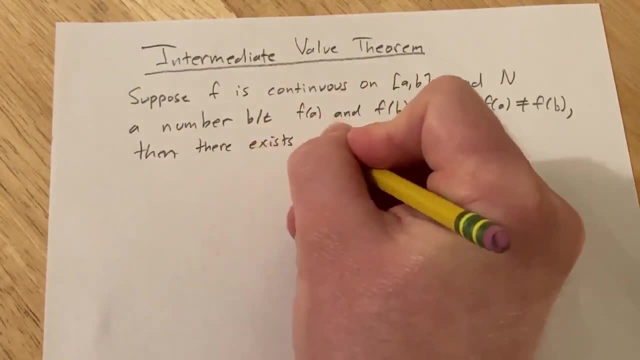 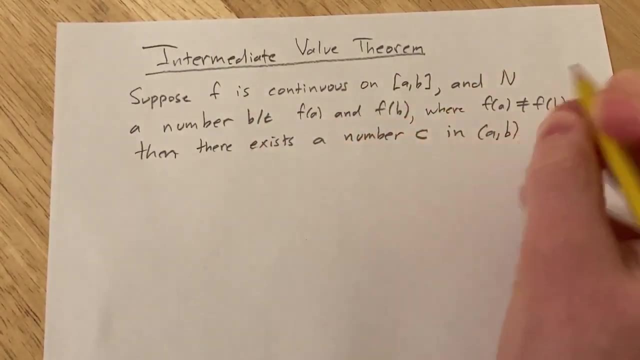 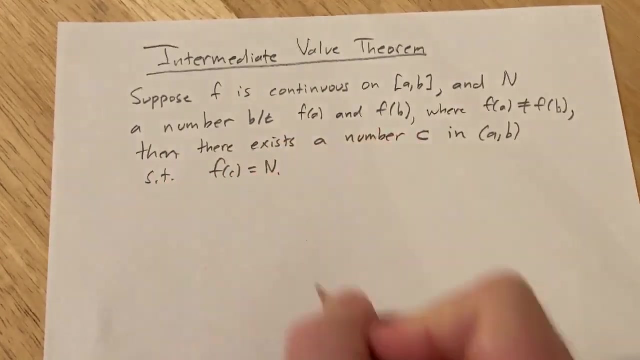 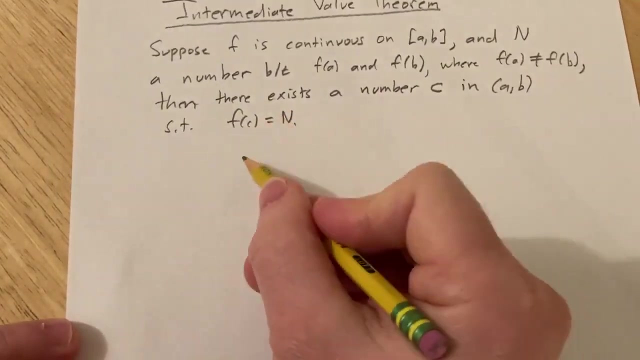 exists a number c in the open interval, so in such that f is equal to n. So when you see it in words like that, it's like: okay, what's going on? what is happening here? let me just give you a quick picture. so this is the y-axis, this will be the x-axis. 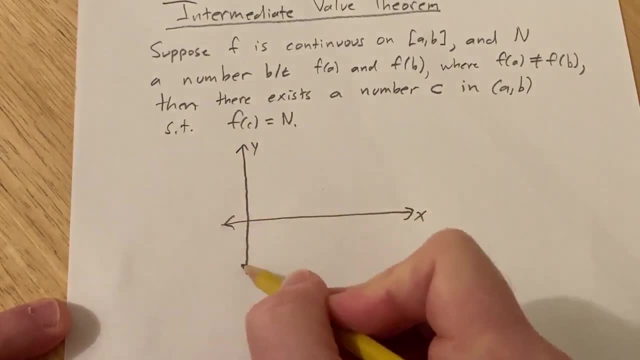 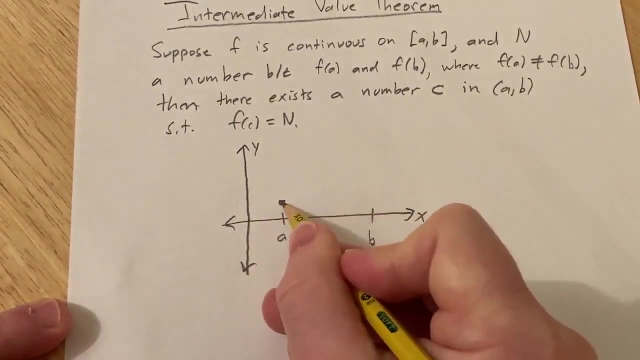 so this is x, this is y, and let's say this is a and this is b, and let's draw a picture of our graph. so let's say we start here and we do this, and so this here would be f of. 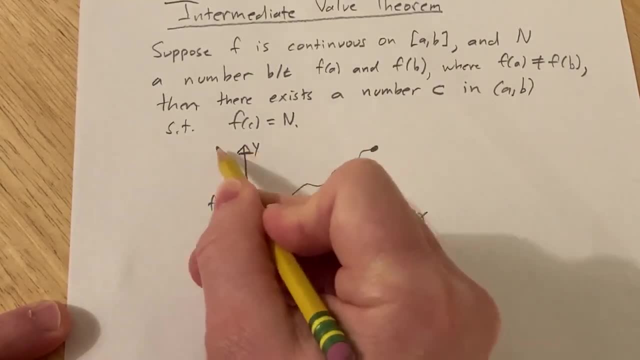 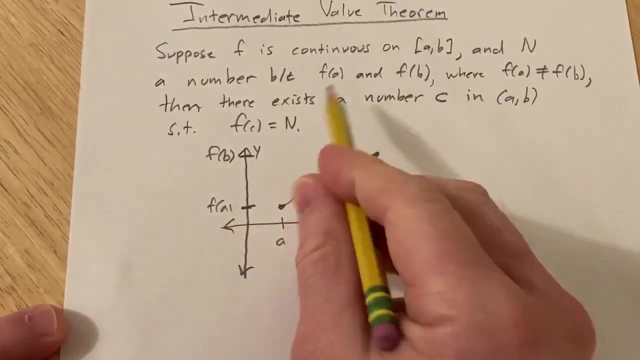 a and this here would be f of b. so we have just a fake continuous function which I just made up and drew. so it's continuous, so it has no holds or breaks. So if you have a continuous function on a- b, which we have here in our beautiful picture, 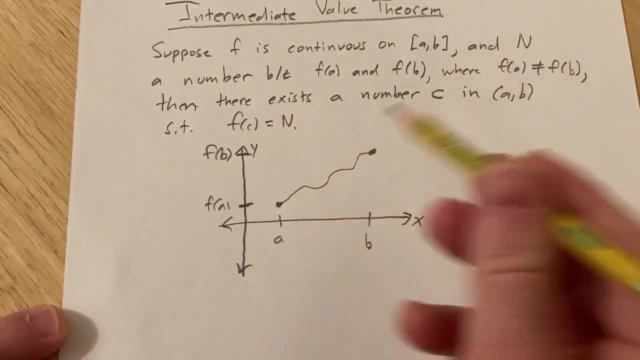 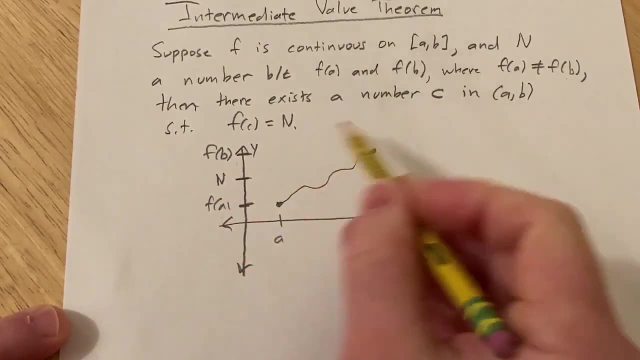 and n is a number between these, and these are different. these are definitely different. so it just basically says, if I pick a number n between these, that there is a number c in the open interval, such that f of c is equal to n, and certainly that's true. 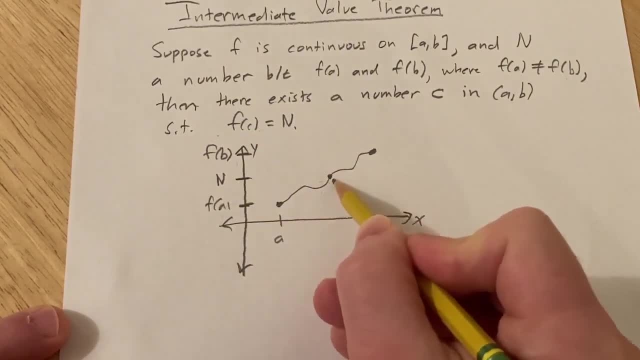 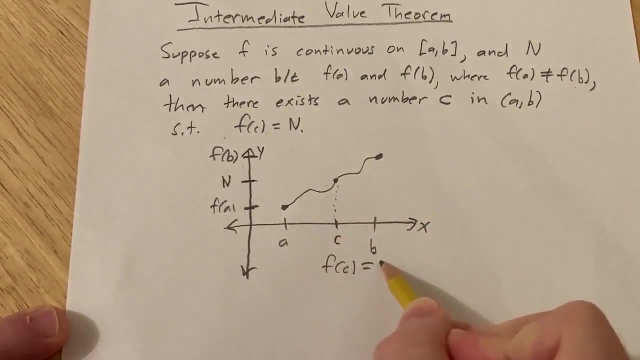 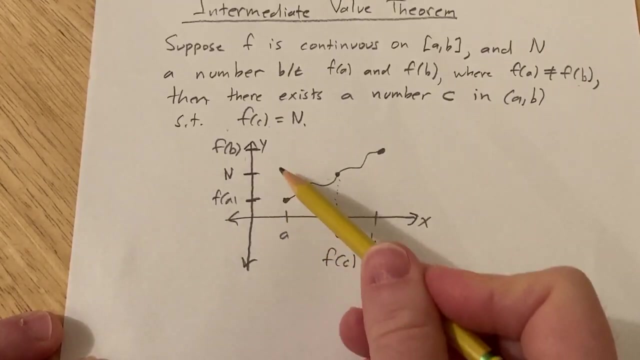 If I pick this n here, this corresponds to this y value and I can find some number c in the interval, such that f of c is equal to n. So it basically says a continuous function on a closed interval takes on every intermediate value. so I can pick any n here. I can pick any value between these and I'm going to 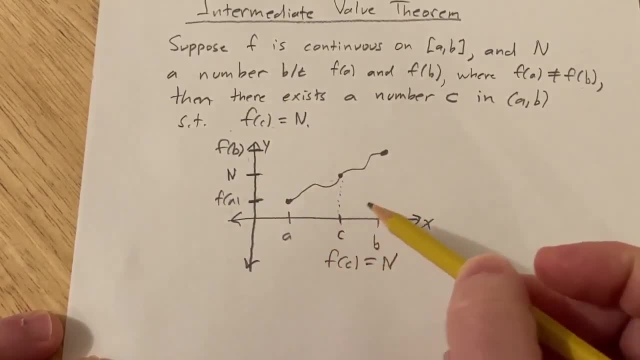 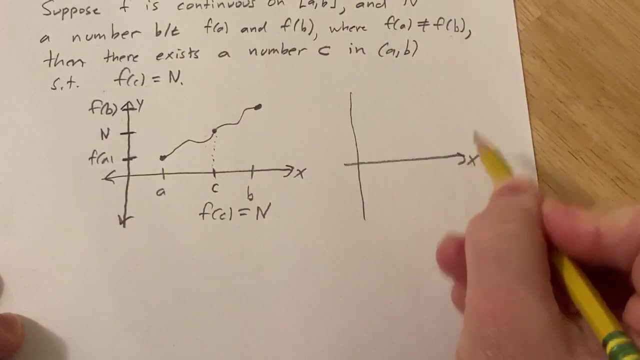 be able to find a number c. Note that in some cases, you'll be able to find more than one number. For example, let's say that I draw that same picture. so again, this is the x-axis, this is the y-axis. 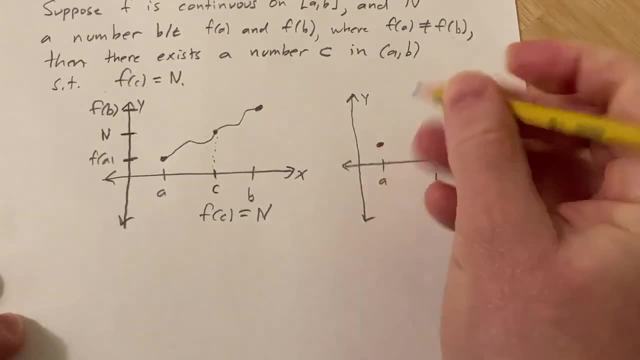 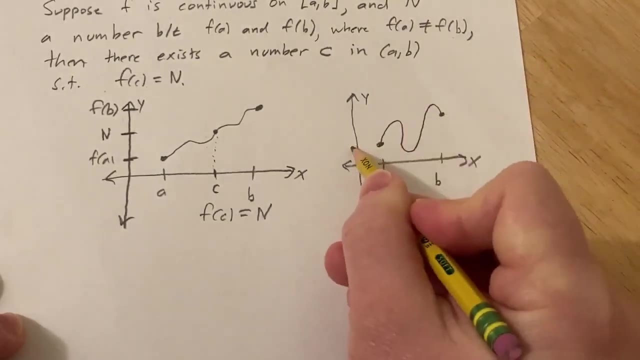 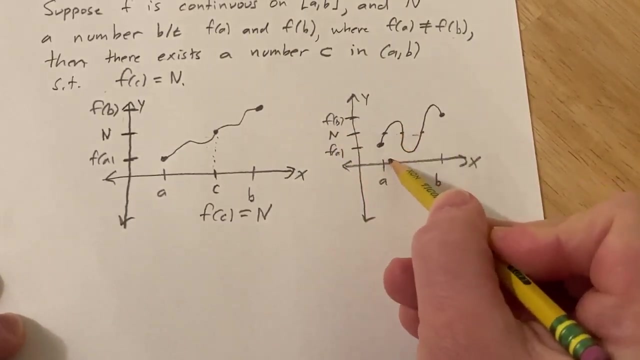 And this is a, This is b, And let's say I do this, Let's say we do something like this, right? So in this case, this is f of a and this would be f of b, And say I pick n here, then I get one, two, three places where I have three different. 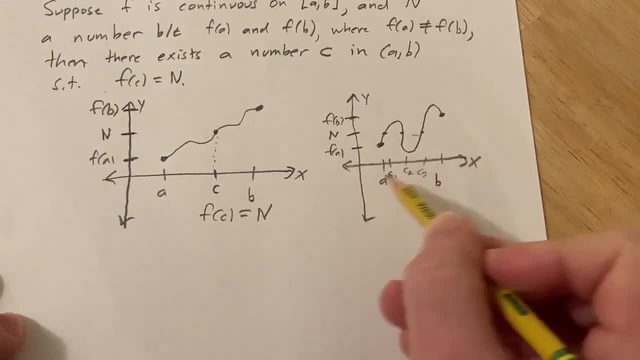 c's. I've got a c1 here, a c2 here and a c3 here. So in this case there's three values of c That give me n. So in this case, f of c1 is equal to n, f of c2 is equal to n, f of c3 is equal to n. 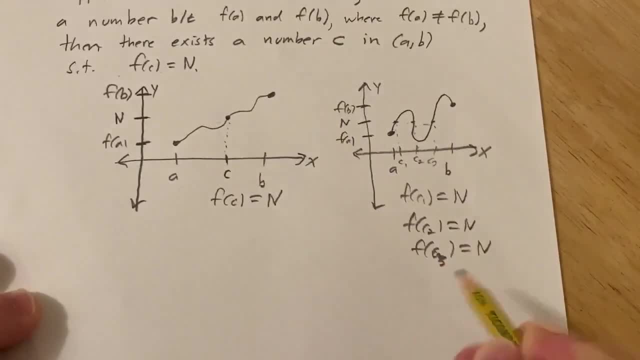 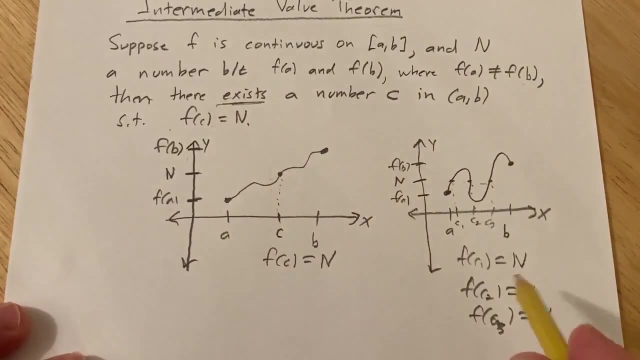 Oops, there we go, c3.. So it doesn't tell you how many numbers there are, it just says there exists. This is called an existence theorem. It also doesn't tell you how to find it, it just tells you that it exists. 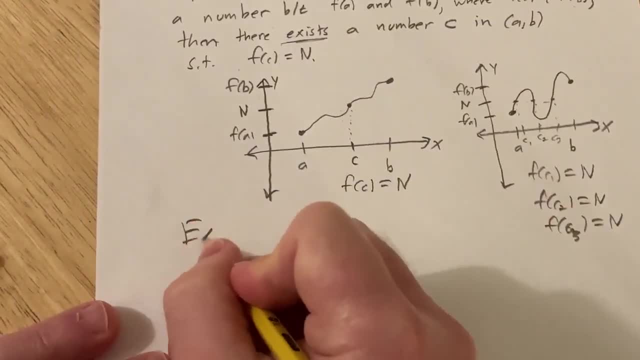 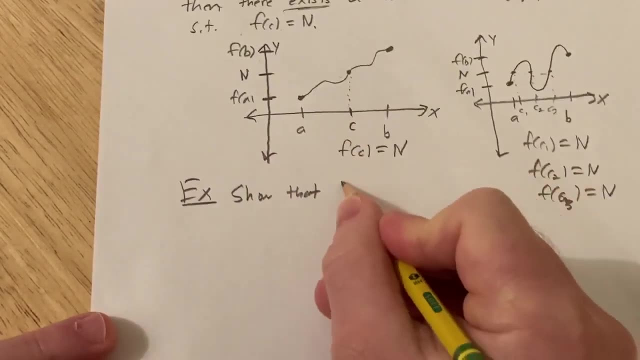 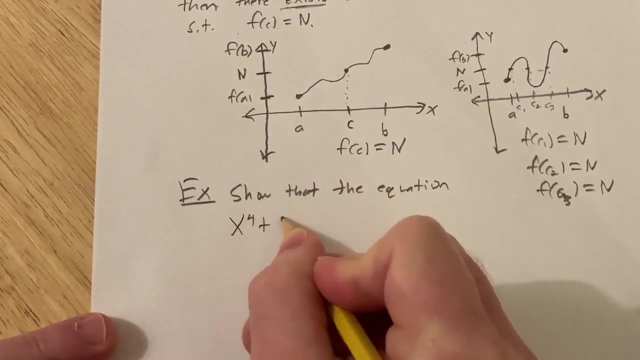 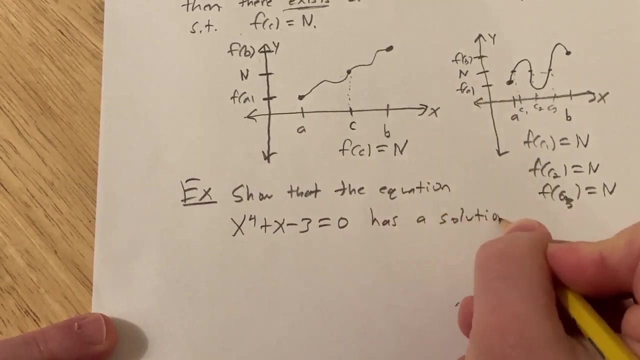 Okay. So let's do an example, Okay, Okay, Okay. And we're just basically going to show that the equation- and let's just say x to the fourth plus x minus three equals zero- has a solution in the interval one two. 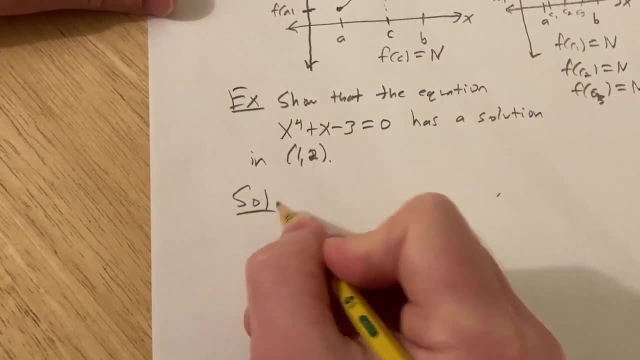 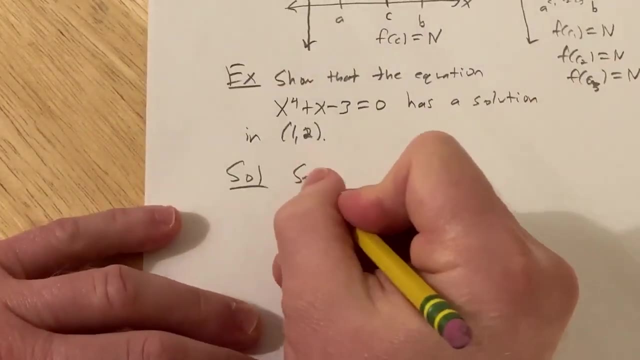 Okay. So solution: We have to basically show that this equation has a solution in this equation. Okay, Okay. So we have to basically show that this equation has a solution in this interval. So to do that, if we want to do it formally, we're going to set f of x equal to the left. 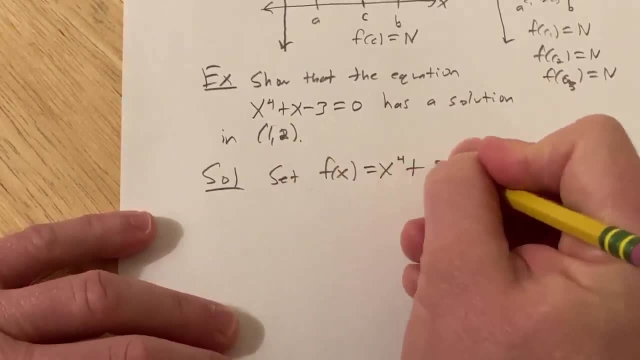 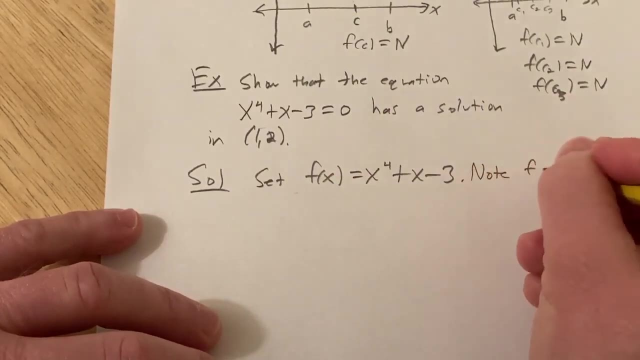 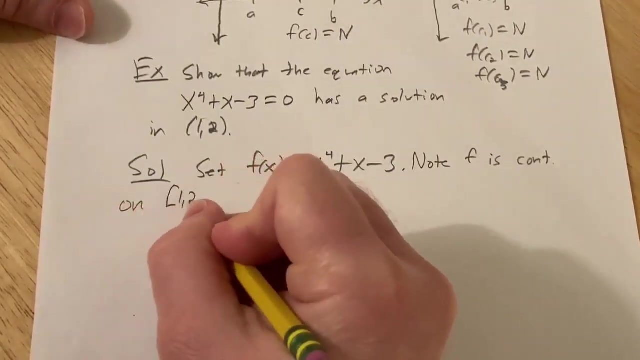 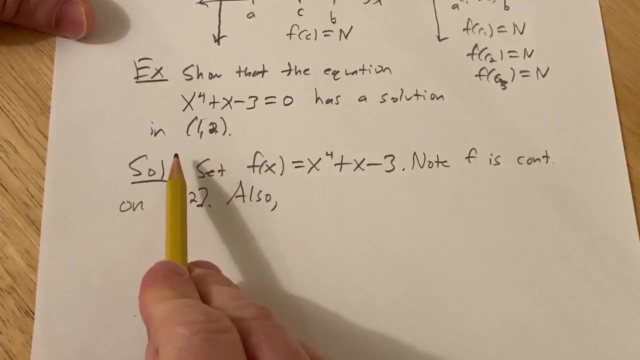 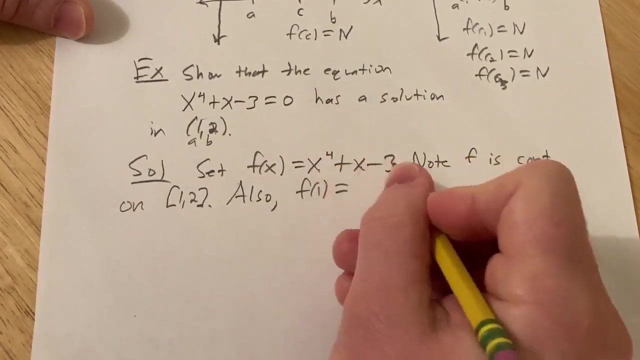 hand side of the equation. So f of x is equal to x to the fourth, plus x minus three. So note this is continuous. Note f is continuous. let's put cont on the closed interval. one, two, Okay, Okay, Okay. 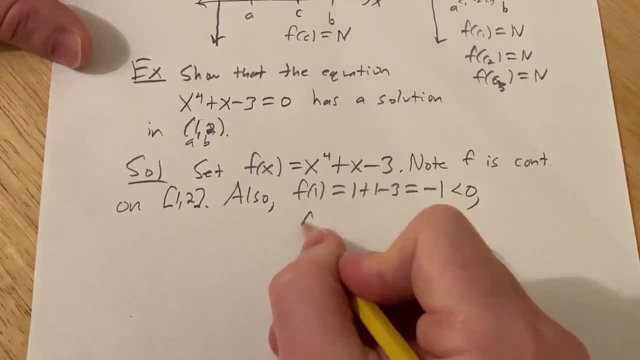 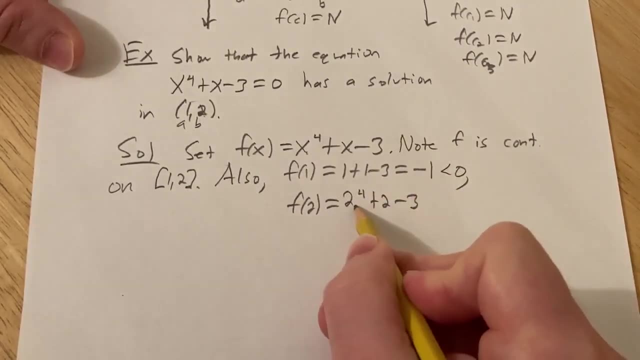 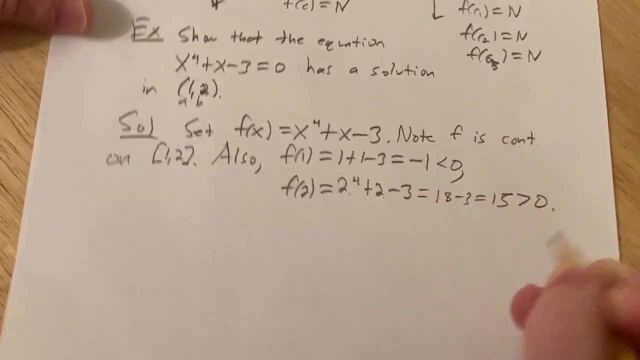 Cool Cool, That's good. Okay, Okay, Cool, Cool, Okay. So you get 18 minus 3,, which is 15,, which is greater than 0.. So 0 is between this number and this number, right? 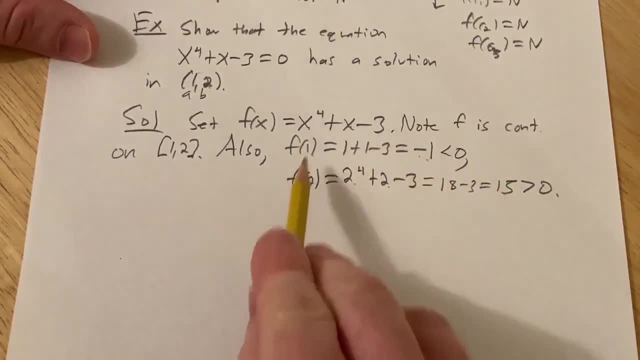 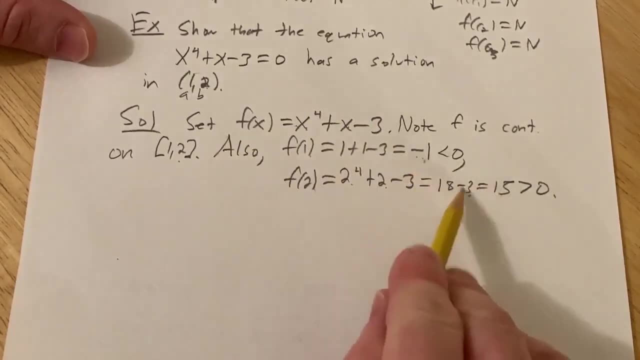 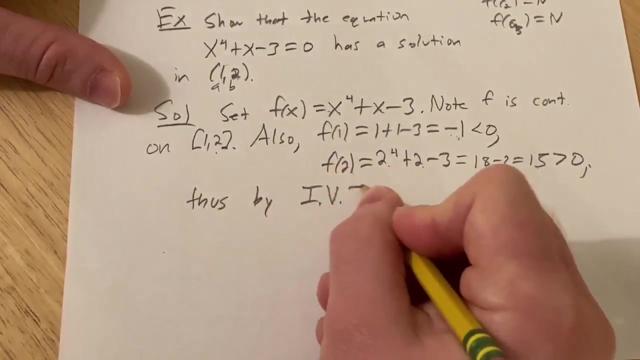 0 is certainly between negative 1 and 15.. And these are different numbers. So we've satisfied all the criteria. We've got a continuous function on our closed interval. These are different and 0 is between these numbers. Thus by IVT, that's the intermediate value theorem. 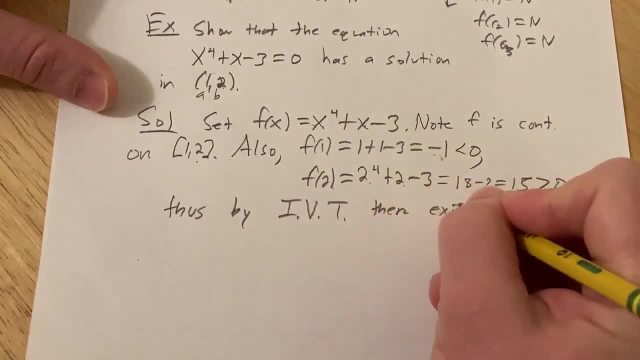 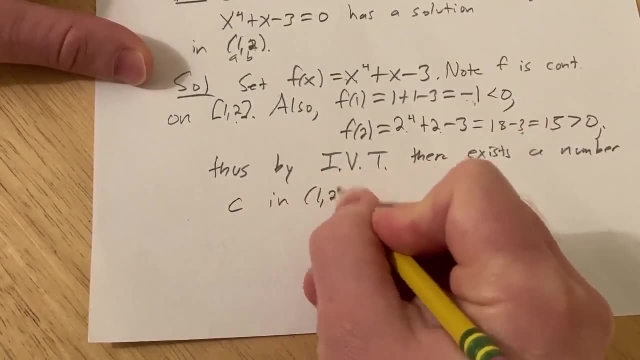 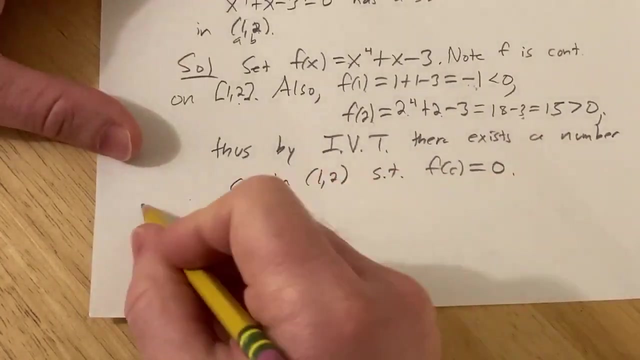 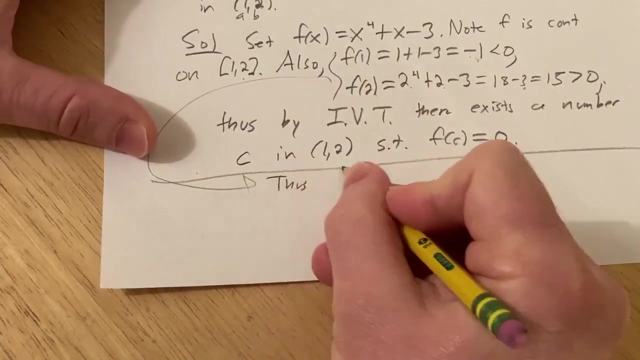 there exists a number c in the open interval, such that f of c is equal to 0. And if you really want to make it match the theorem, you could say something else here. From here you could say thus: f is continuous on AB. 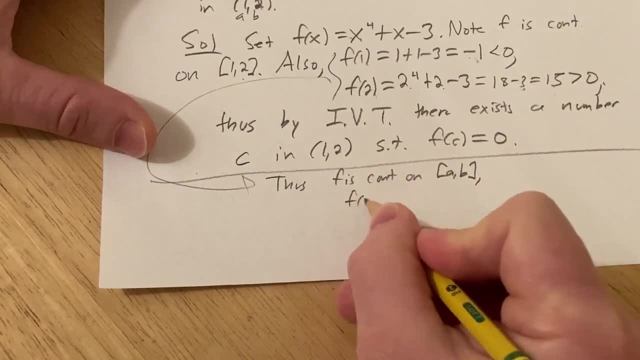 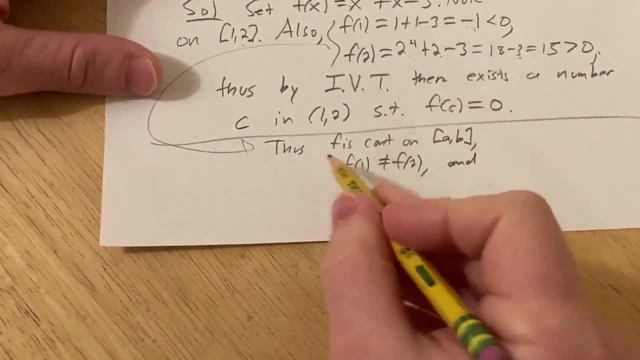 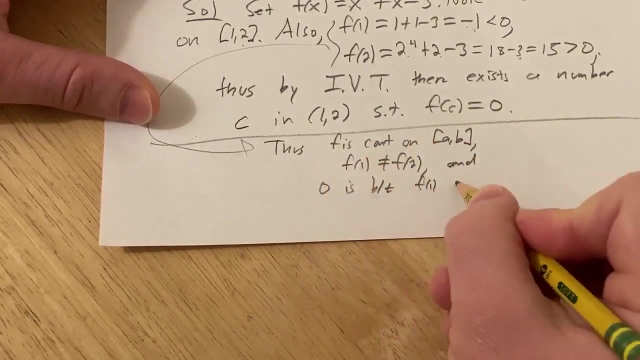 f of 1 is not equal to f of 2.. And so, if you want to elaborate and make a better solution, you would say this, this, and then you would reiterate, You would say: and 0 is between f of 1 and f of 2.. 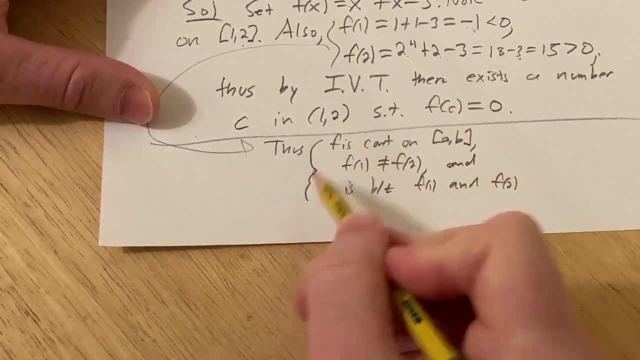 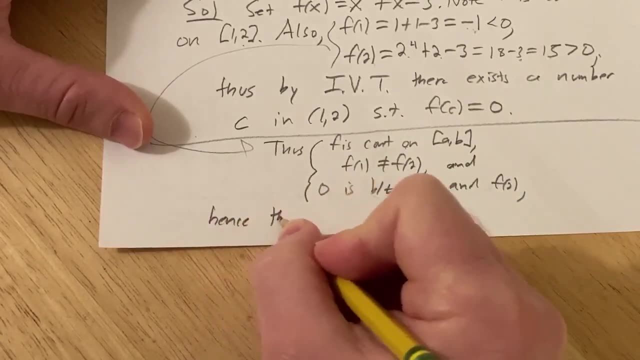 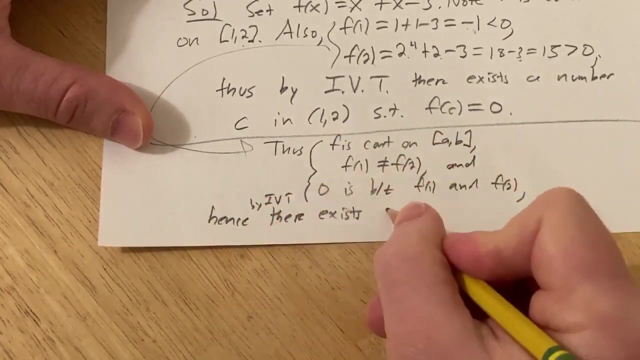 So these are the things we're using, right? So all three of these things imply there exists a number c. Then you would say: hence there exists. hence, by IVT, there exists c in 1, 2, such that f of c is equal to 0..